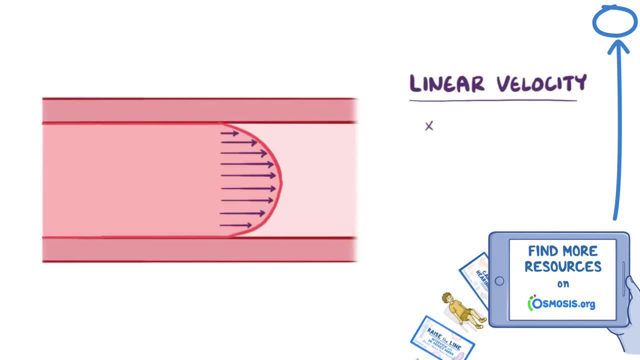 velocity of the blood, which is how fast it's moving in a straight line, is greatest in the center of the blood vessel and lowest near the walls of the vessel, dropping to zero at the wall. Sometimes, though, blood flow is disrupted, like if it has to pass. 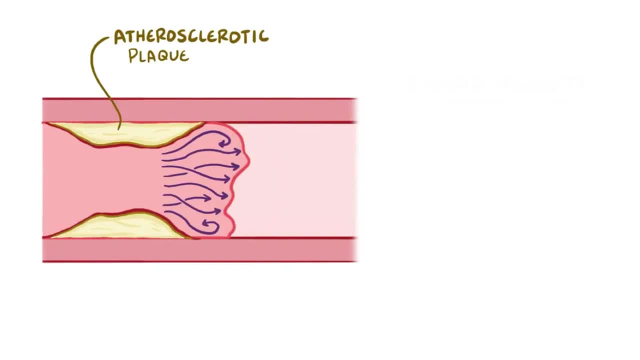 by a crusty old atherosclerotic plaque. Subtitles by the Amaraorg community. Now, there are a number of factors that help predict turbulence, and they include the density of the blood, usually written by the Greek letter rho, as well as the viscosity of the 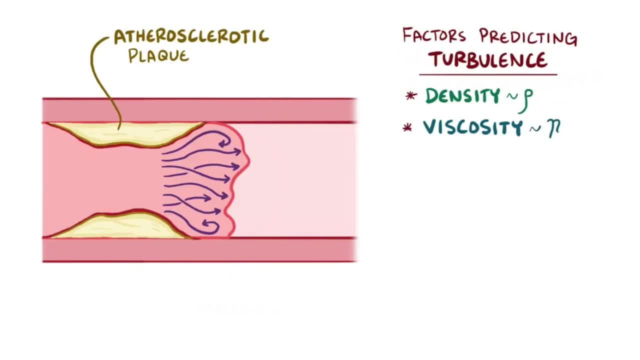 blood, denoted by the Greek letter eta. You can think of a fluid's viscosity as kind of like: its thickness- like, for example, the viscosity of honey- is a lot greater than that of water. After that there's the velocity of blood flow, or just V, and then finally there's 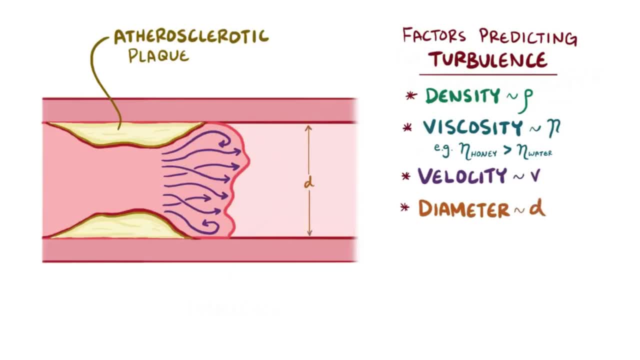 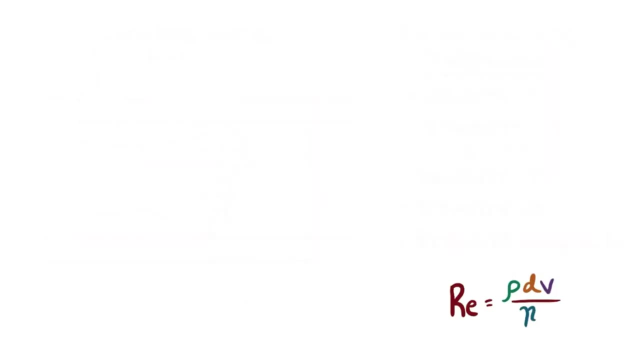 the diameter of the blood vessel or d. These can all be used to come up with a single value, the Reynolds number, and the equation goes like this: Reynolds number equals density times diameter, times velocity, all over viscosity. Generally speaking, if the Reynolds number is low, below about 2000,, then blood flow. 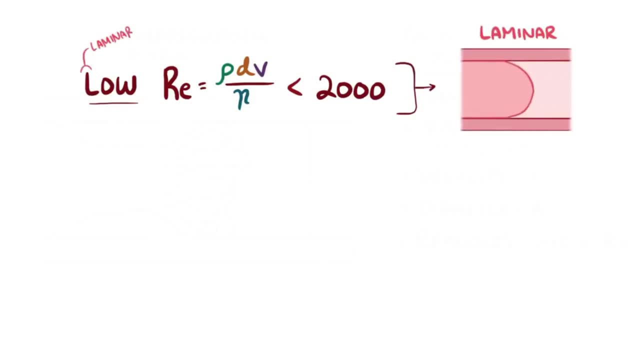 will be laminar. Think of the diameter of the vessel as the diameter of the vessel. think L for low and L for laminar. But if the Reynolds number is above 3000, it'll likely be turbulent. A Reynolds number between 2000 and 3000 is somewhere in between. 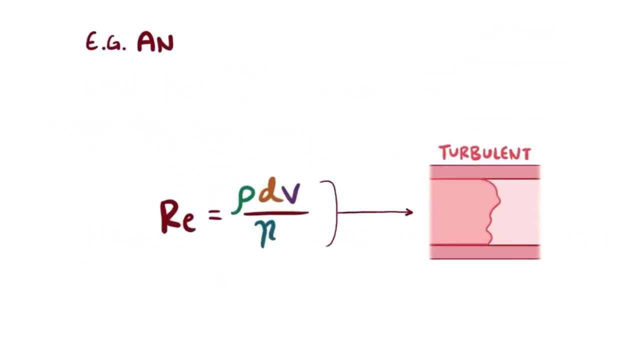 As a real life example of turbulent blood flow. a person with anemia has a low red blood cell count and in general has a lower hematocrit, which is the ratio of the volume of red blood cells to the total blood volume. This essentially means that the blood is less thick or viscous. 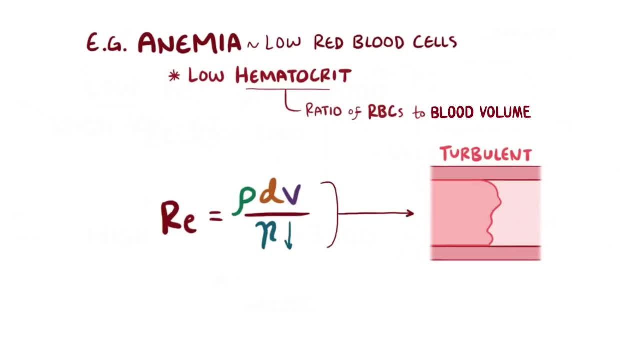 Based on the equation: if viscosity decreases, that means Reynolds number increases. Also, these individuals often have an increased cardiac output, which means increased blood velocity and therefore increased Reynolds number. Now, another example would be a person with a thrombus or a blood clot, which just like 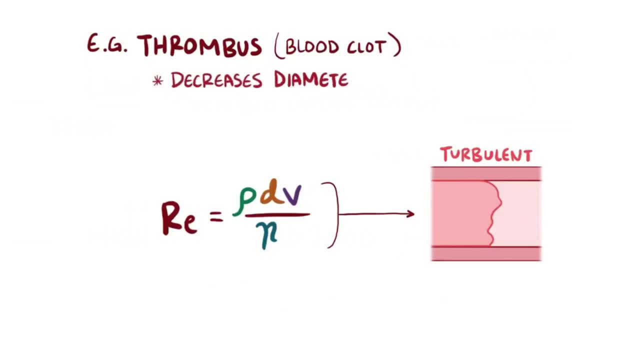 atherosclerotic plaque would narrow or decrease the diameter of a blood vessel. Now at first glance this seems a little weird. huh, decrease in diameter should probably decrease Reynolds number. but it turns out that the blood velocity also depends on the diameter of the vessel. by the equation velocity equals. 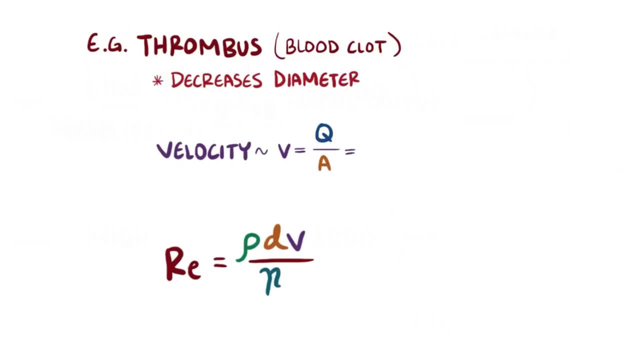 flow rate q over area where the area is the area of a circle, which is pi times d over 2 squared, and this comes out to be 4q over pi d squared. Taking that guy and plugging it in for velocity, we now see that as the diameter decreases, Reynolds number increases. 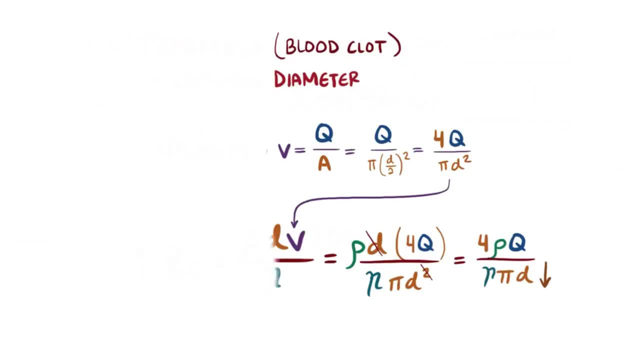 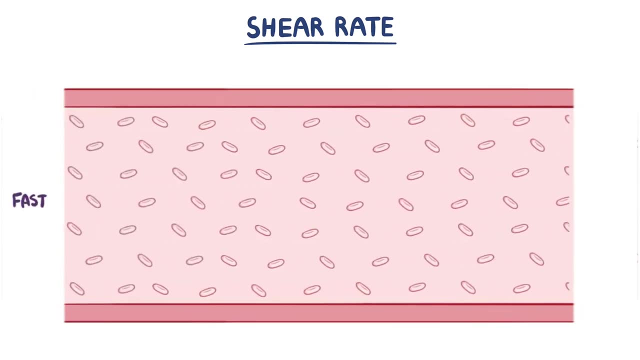 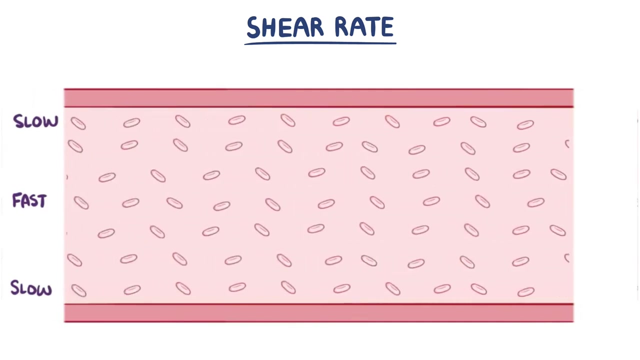 Now, a related concept is shear rate, and remember that blood velocity depends on whether it's in the middle, which is where it's the fastest, or it's near the walls, where it's the slowest. In fact, at the molecular level, just outside the walls, water molecules. 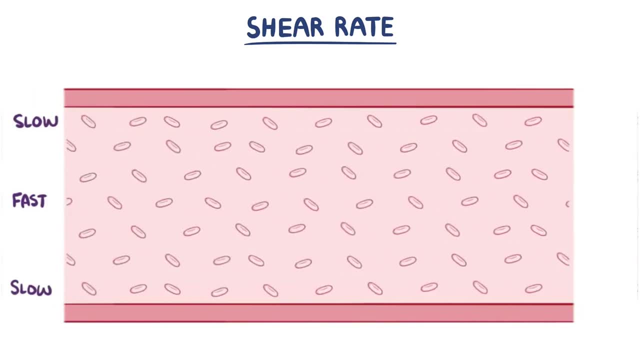 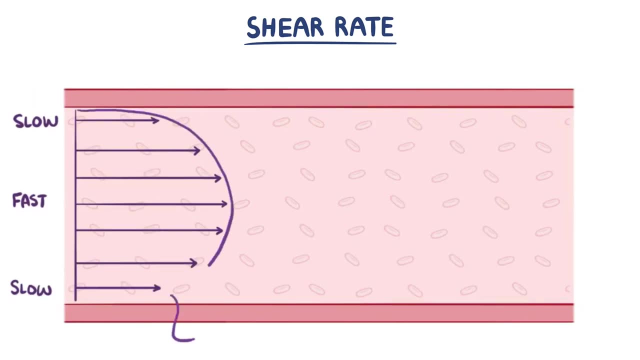 are just sort of sitting still and not moving, And if we freeze the velocity of the vessel, we're going to see that the velocity of the vessel is actually very low. If we freeze this and then plot those velocities, we'll notice that the difference between adjacent velocities is parabolic, meaning that, as you 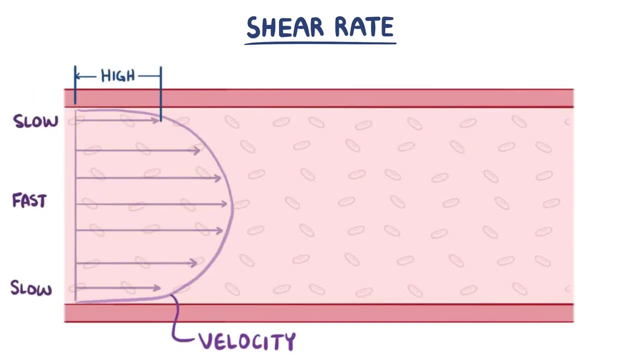 move away from the walls, velocity at first jumps up pretty quick, but as you get near the middle the change in velocity is actually pretty low. This difference in relative velocities is the shear rate. So if we wanted to plot shear rate near the wall, where velocity is. 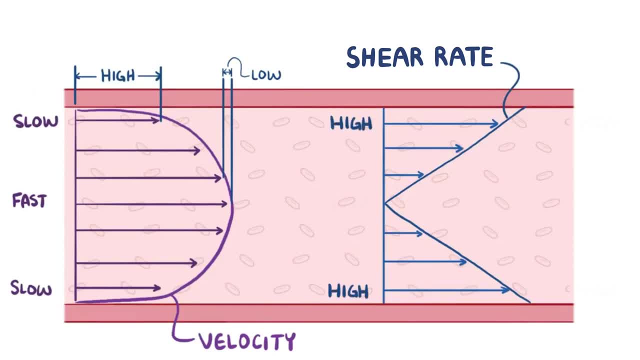 changing the most. shear rate's actually the highest and in the middle shear rate is very low and actually decreases. Shear rate goes hand in hand with viscosity, because the higher the shear rate, the lower the viscosity of the blood. This is because shear, or simply the differential velocities. 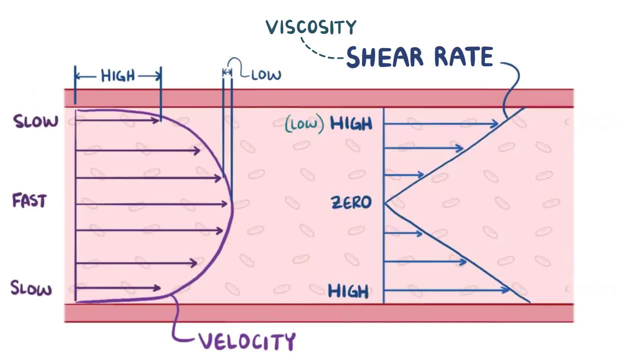 helps to pull the elements in the blood apart, decreasing its stickiness or viscosity, making blood less viscous at the vessel walls and more viscous in the middle of the vessel. Now let's say that all that blood's somehow moving at the same velocity and we're going. 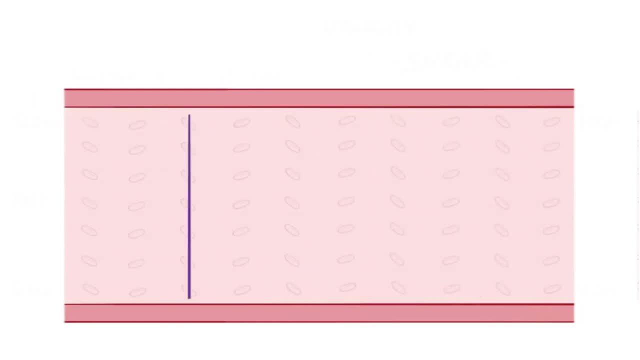 to get the same velocity. Well, in that case, if you plot it out, there's no change in velocity across the blood vessel, and that makes plotting shear rates pretty easy. since there's no change in velocity, there's no shear rate, and likewise this fluid isn't.